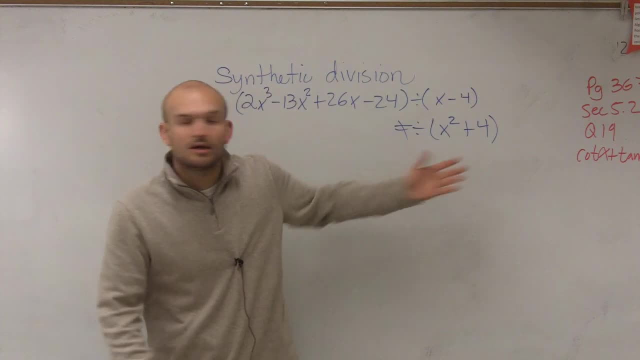 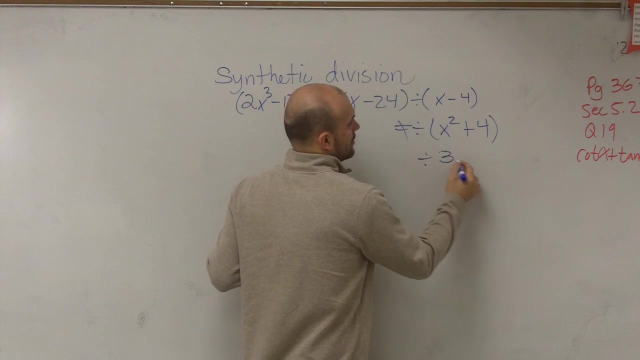 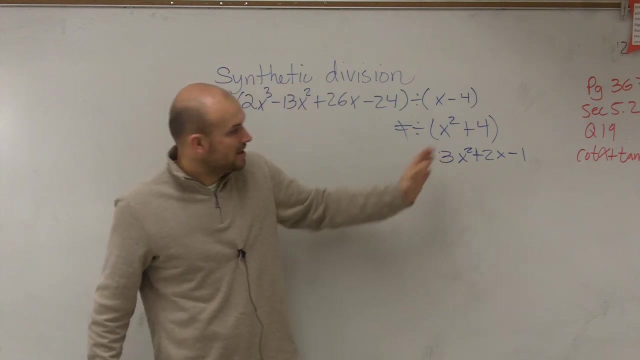 Okay, you cannot divide by, because that's not linear. right, That's quadratic. You also cannot do. you could also not do like a 3x squared plus 2x minus one. Again, that's quadratic. It's not linear form. But there's three terms. right, It has to be a linear binomial, which we're going to talk about a little bit further in here. So as long as you have it in linear form, you can divide using synthetic division. 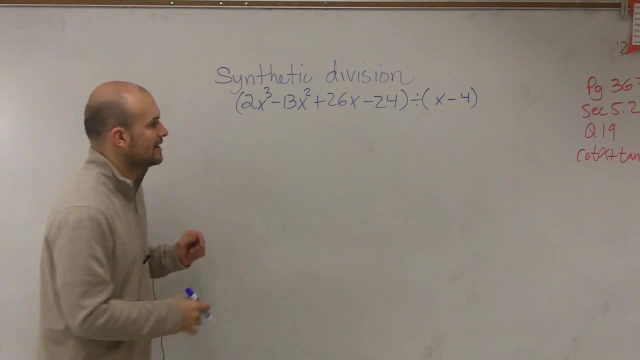 Now the next thing that we're going to do- when using synthetic division, all right- is you have to make sure that your dividend is in standard form, meaning you have it in descending order with your largest degree first and then in descending order from there, All right. So what we're going to do is we're going to create a box And all we're simply going to do is take the coefficients of each term and put them into the box, kind of like on their own column. 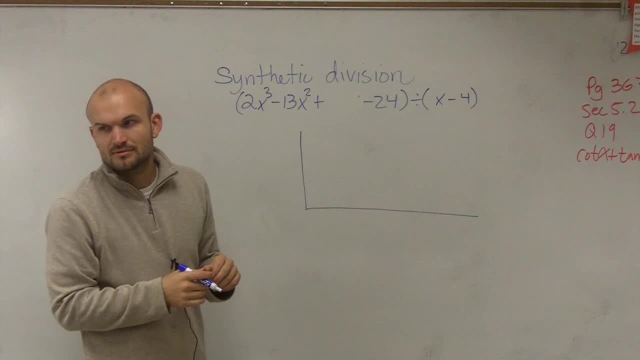 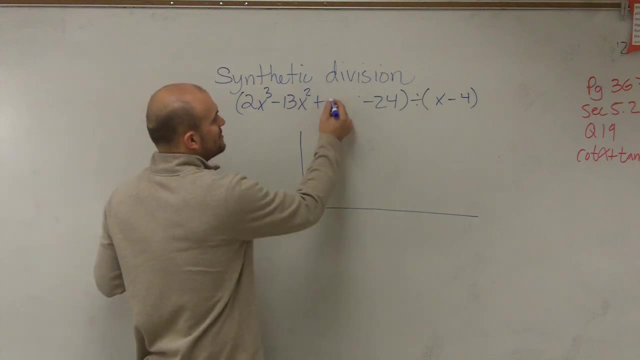 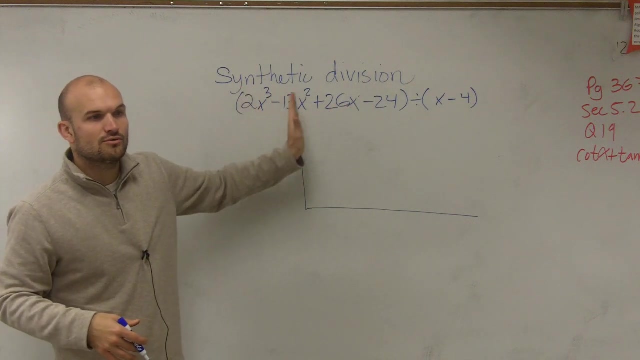 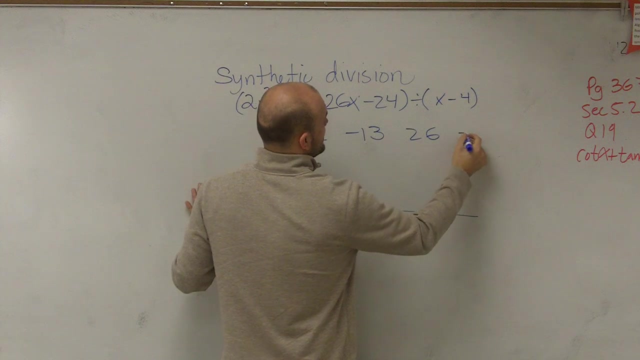 So let's pretend there was not an x here. That was 26,. right, Okay, Let's pretend there wasn't an x here. If there was no x there, you'd want to put a zero in for its place. All right, But we do have an x, so we're going to write 26x. What I'm saying is, if there wasn't one, you'd make sure you put a zero, But for every variable you want to make sure that you have a place value. So therefore, I have 2, negative 13,, 26, and negative 24.. 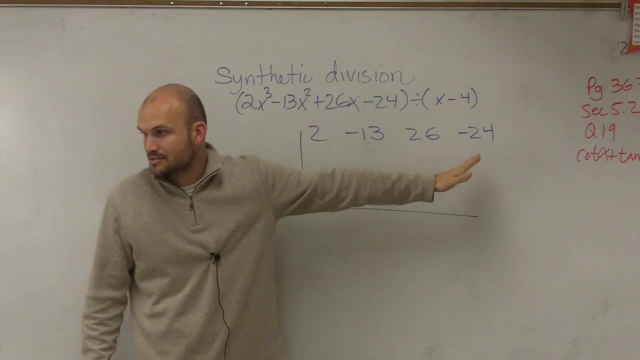 So you're going to take the coefficient of each term and you write them inside the box. All right. Now negative 24 is a constant. You're right, It's not a coefficient, It's a constant. But you're going to include the constant as well. 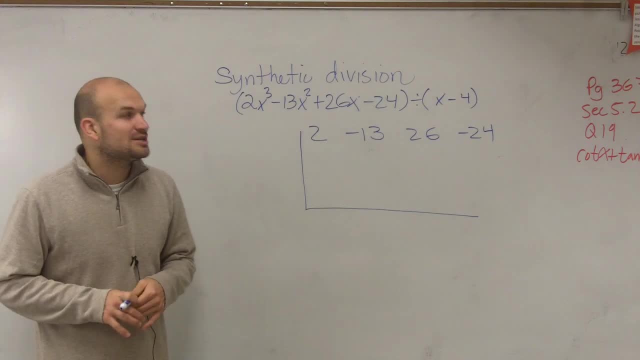 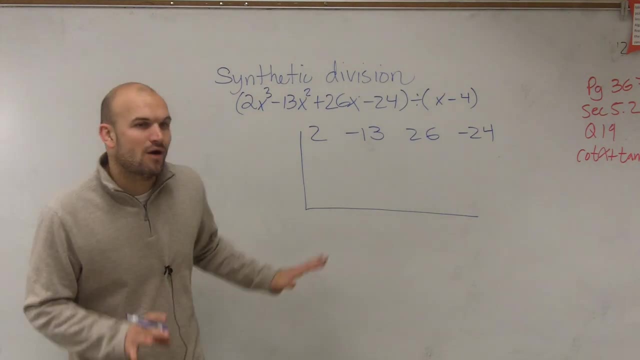 Then, Justin, the next thing you're going to do now. ladies and gentlemen, I'm not going to get too much into this. all right, because we're going to learn about what this is later, But for right now, all I want you guys to focus on is just taking the opposite of what you're going to do. 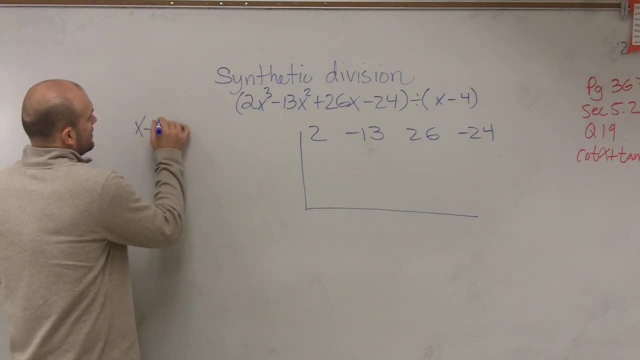 That's in your actually. well, you can just take this. The easiest way to do it is just to take whatever your divisor is, set your divisor equal to zero and solve. That is going to be the number you're going to be dividing by as your divisor. Okay, We'll explain a little bit more about that later. We'll learn why. is it the positive 4.? 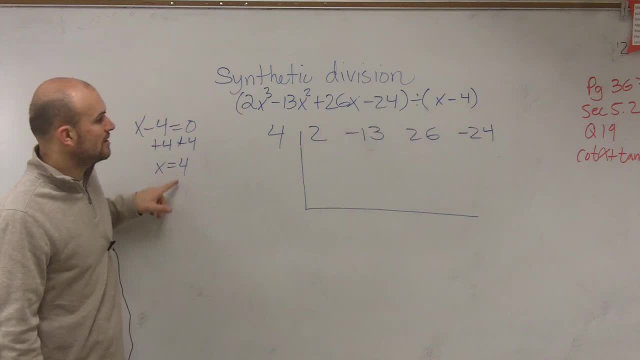 For right now. just take your divisor, set it equal to zero, and that's going to be what you're going to use for your synthetic division. Okay, So here's the process. It's very basic. I'll leave it up here as you guys practice. It's pretty easy to kind of follow. 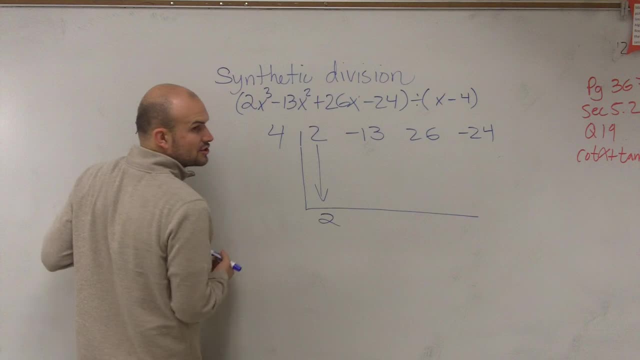 First number is a freebie. You bring it down, which is your 2.. Then you multiply 2 times, 4 is 8.. Then you add Negative. 13 plus 8 is going to be a negative 5.. 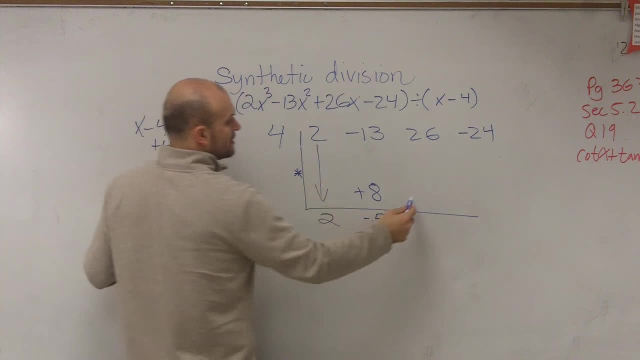 Then you multiply Negative 5 times 4 is a negative 20.. Add 6 plus a negative, 20 is going to be now a positive 6.. Multiply 6 times 4, positive 24.. Add Negative 24 plus 24 is a zero. 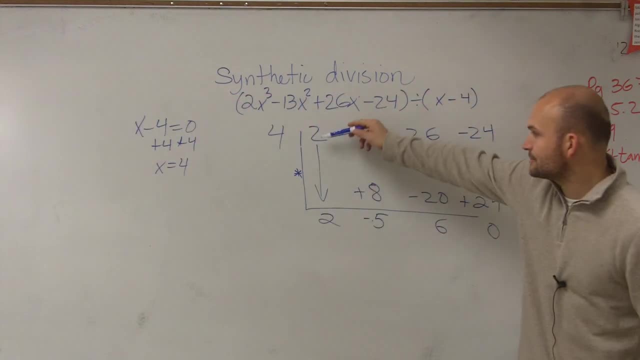 Sure. So all we do first one is a freebie, Bring it down. Multiply 2 times 4 is 8.. Add Negative: 13 plus 8 is negative 5.. Multiply Negative 5. 5 times 4 is negative 20.. Add Positive 26 plus a negative 20, positive 6.. Multiply 6 times 4 is positive 24.. Negative 24 plus 24 is zero. 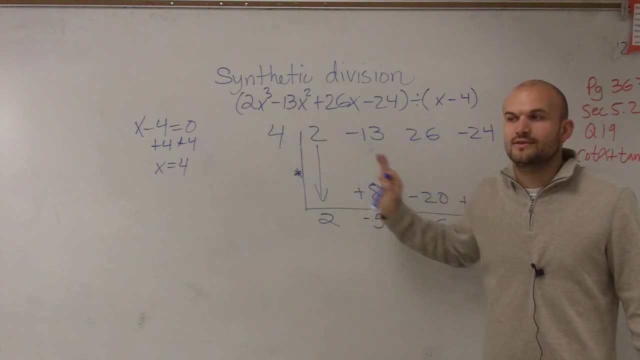 The one sometimes we like to think about. it is when you go in the vertical or the not vertical. but when you go diagonal lines, you multiply. When you go vertically, you're adding. Yes, Are you allowed to use this for a long term? just to say: 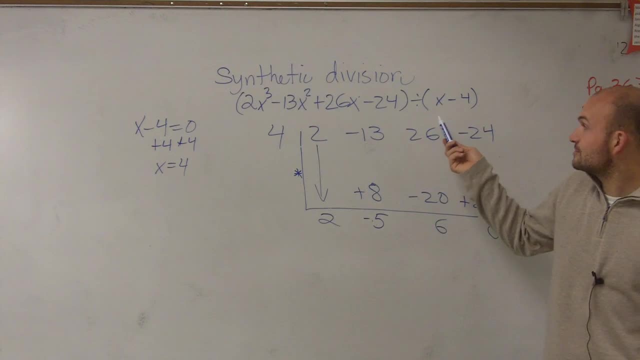 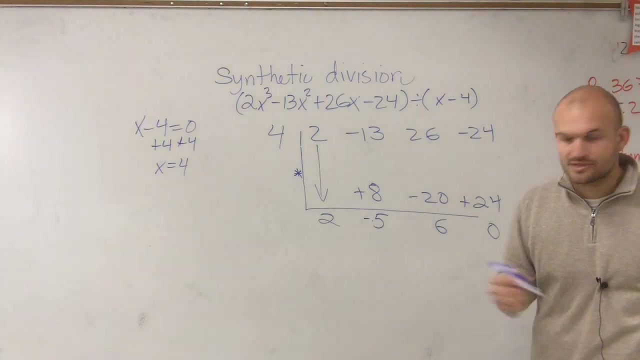 Yes, But you only when you're using long division, when you're dividing by a linear binomial. Okay. However, for your test, I will ask to see long division and I will ask to see synthetic division. So the last step to get your answer is sometimes. this is the best way I like to explain it.